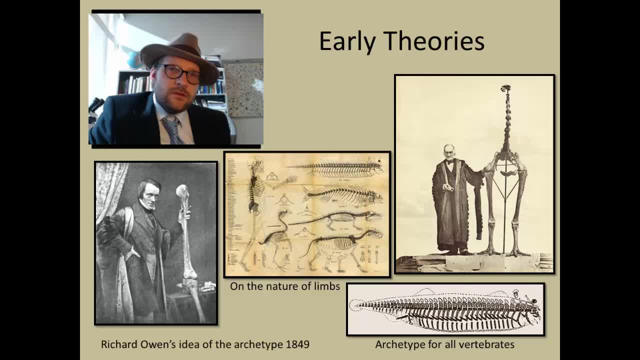 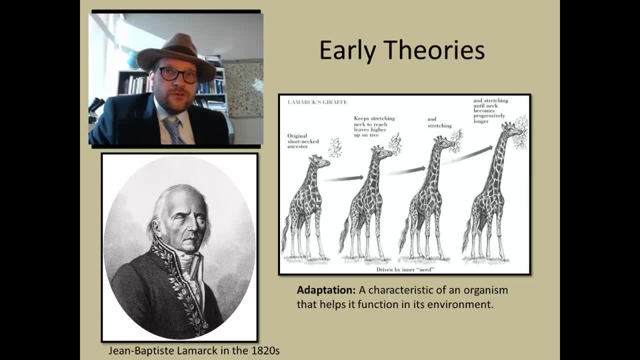 the similarities between organisms and suggesting some sort of relationship. One of the earliest people to invoke the idea that species change was Jean-Baptiste Lamarck. Lamarck was of importance in this course because he coined the term invertebrate. Lamarck started out as a botanist studying plants at the poorly funded Paris Botanical 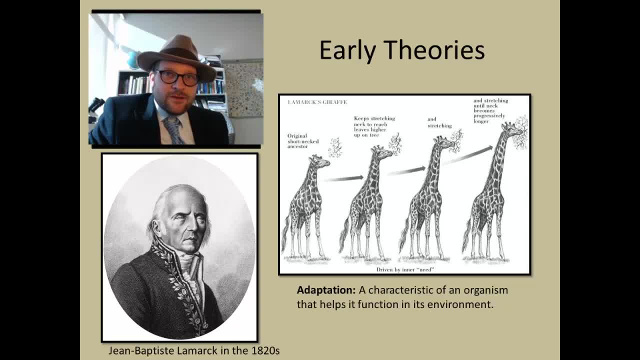 Gardens as an unpaid student working part time as a clerk, spending as much time as he could on describing plants. In 1793, Louis XVI and Marie Antoinette were executed and the new post-revolutionary French government went on to engage citizens with science and, as such, helped form the Musée. 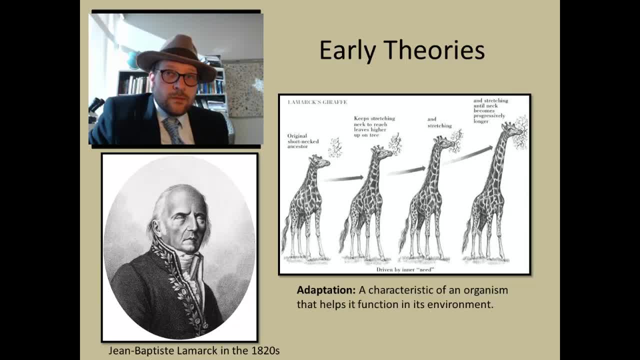 National de l'Historie Naturelle Natural History Museum and Natural History in Paris, Lamarck was appointed to the curator of insects and worms. Despite not knowing much about insects and worms, Lamarck became fascinated with them and coined the term invertebrate. 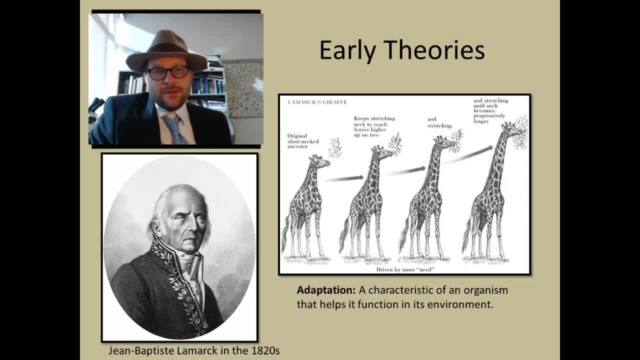 Lamarck was at the time a student of everything, and he came to recognize great things, such that all life is composed of individual cells. He also helped divide invertebrates into the groups that we will be studying in the coming lectures. But he also, in 1809, proposed that species, particularly animals, could change over time. 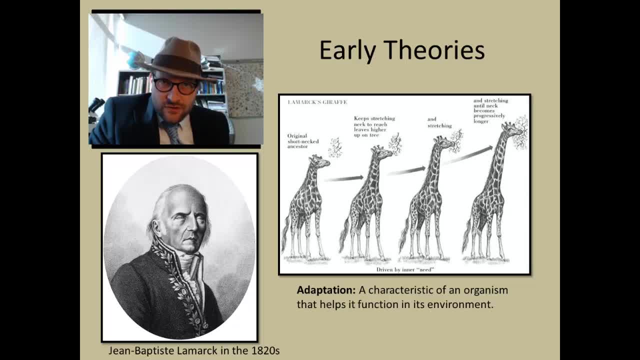 Specifically other裡面 what i will also highlight, the Weber's other examples of 20 different kinda methods to manage invertebrates. Selecting an adorable little five-feet-tall mushroom would use the absolute number of pointer and a emphasis inSpec. This was as stated as follows: All acquisitions or losses wrought by nature on individuals through the influence of the environment in which the race has long been placed, and hence doing that to influence the predominant use of permanent or permanent disuse of any organ, All of these are preserved by the reproduction to new individuals which arise如果 ernst. 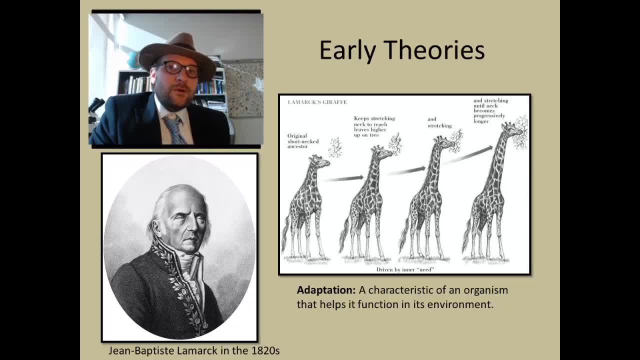 Stellen auf corpo, statt unter AllerOMarcusYer higherff shirt- esex. http// catches'mapnet. The common example that is invoked in how Lamarck viewed evolution is the giraffe. Lamarck viewed the influence of the environment would extend to the giraffe's neck and 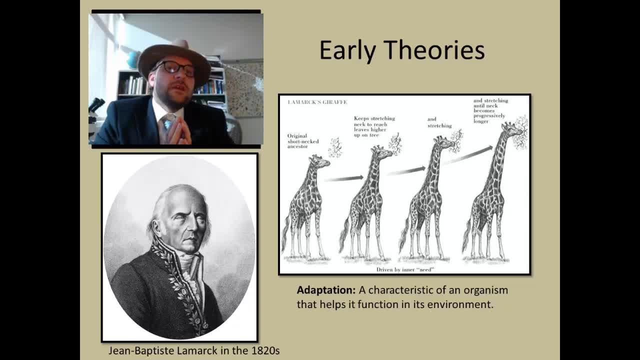 it would cause it to reach for higher and taller trees, and that this acquired inheritance was then passed on to the offspring. Hence often his ideas called acquired inheritance. Once more important was Lamarck's visionary idea of adaptation: that organisms have characteristics that help them function in the environment they live within. 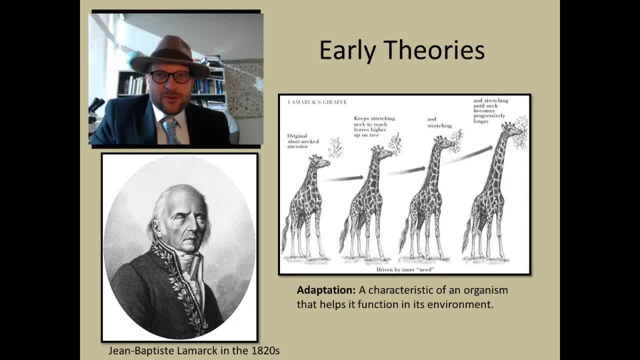 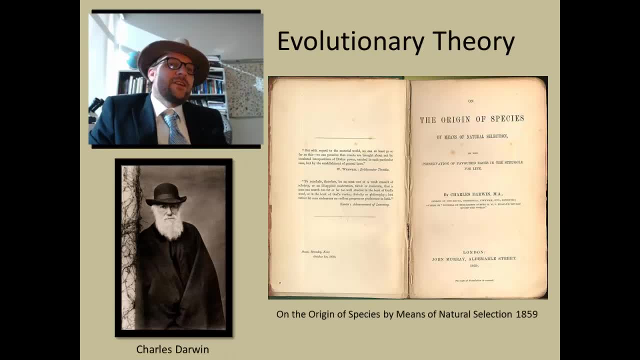 At the end of Lamarck's life he became blind and that is when this portrait was made of him. Sadly, he died 30 years before Charles Darwin published his Origin of Species. Every introductory biology course goes into detail about the work of Charles Darwin. 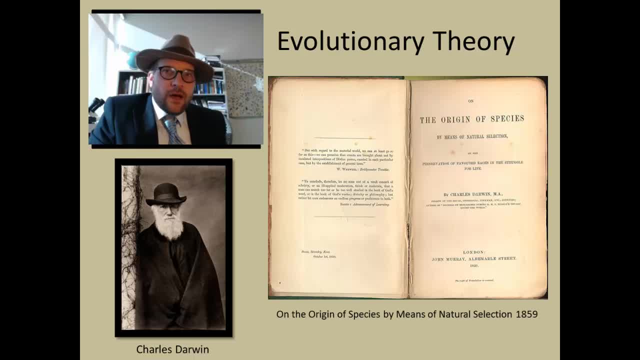 Though Darwin collected fossils on his journey around the world, his fossils were given over to the British. Hence fossils did not occupy a major portion of the book on the origin of species by means of natural selection. In fact, Darwin lamented the poor state of the fossil record and much more of the book. 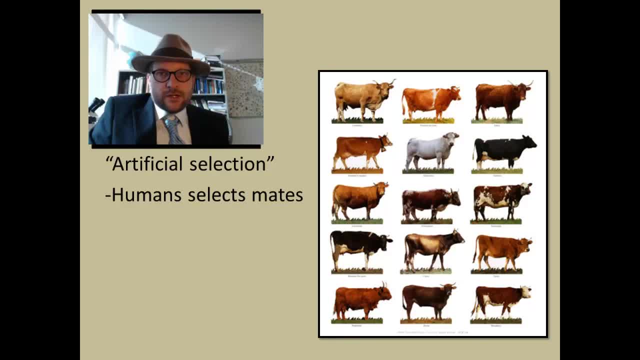 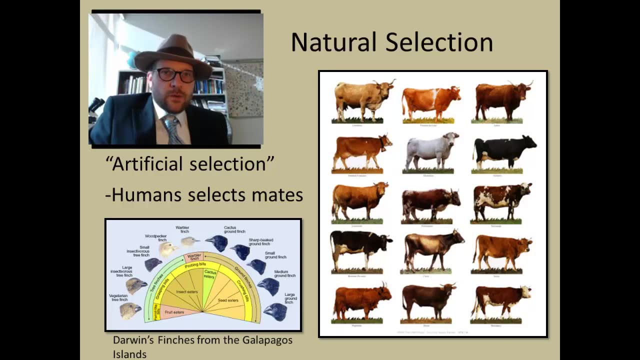 was detailing the discussion of artificial selection or selective breeding. Much of Darwin's ideas came from his passion to raise different domestic animals and plants and breeding them for desirable traits. What Darwin wondered Is if this selective breeding was occurring naturally, for example in the finches he collected. 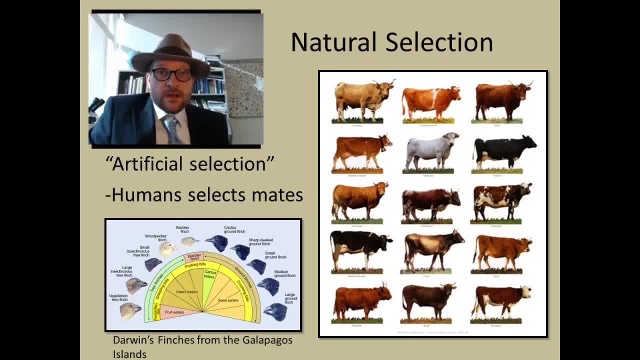 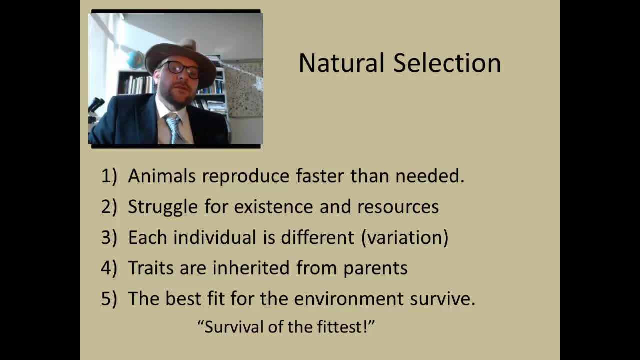 in the Galapagos Islands, And this is his idea of natural selection. Darwin's theory of natural selection can be broken into five key ideas. Animals reproduce faster than needed. There is a struggle for existence and resources, Each individual is different and there is variation in the population. 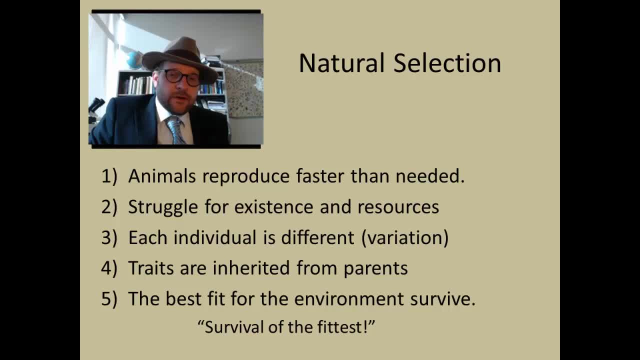 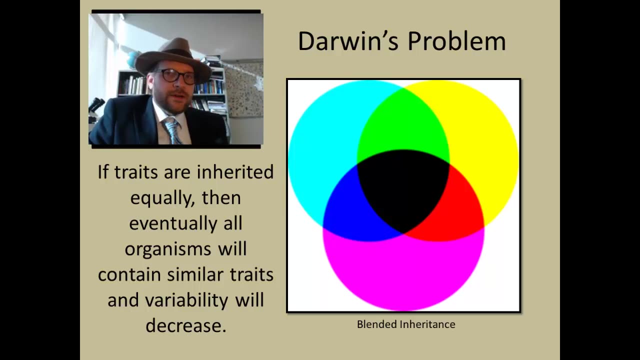 Traits are inherited from parents, and the best fit for the environment are the ones that survive. Darwin, however, had a big problem with this theory. If traits are inherited equally, then eventually all organisms will contain similar traits and variability will decrease. This is referred to as blended inheritance. 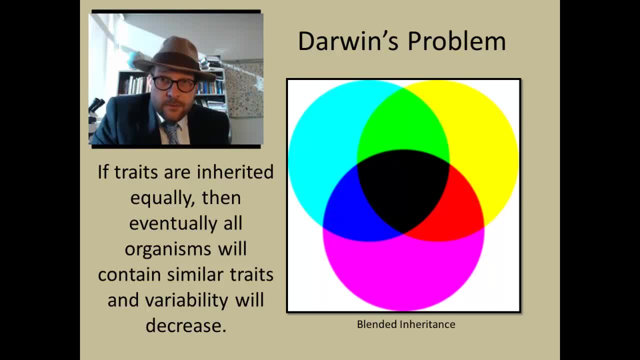 Blended inheritance is what happens when you mix colors together. if you have two individual organisms and they mate, And the resulting offspring exhibit a blend of characters from both parents. As each generation is born, the variation of the colors will decrease until all individuals. 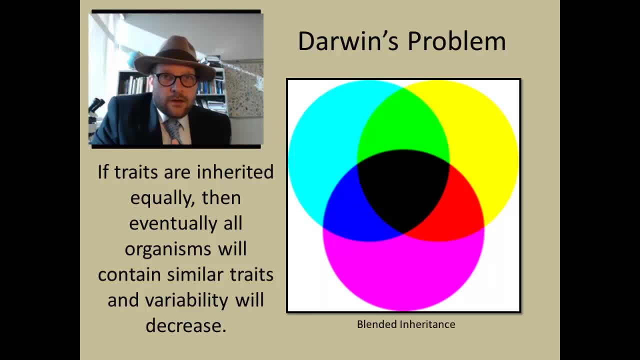 will look the same. They would all be black in color. There had to be a way to introduce new variation within the population. Where did this variation of traits in a population come from? Ideas were wild and crazy. From mutation, Such as the hopeful monster hypothesis of Goldsmith in the early 1900s. 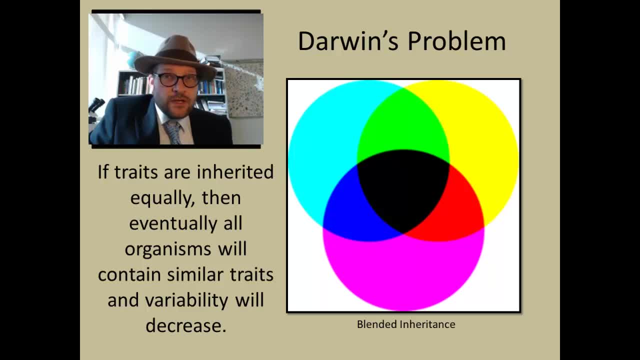 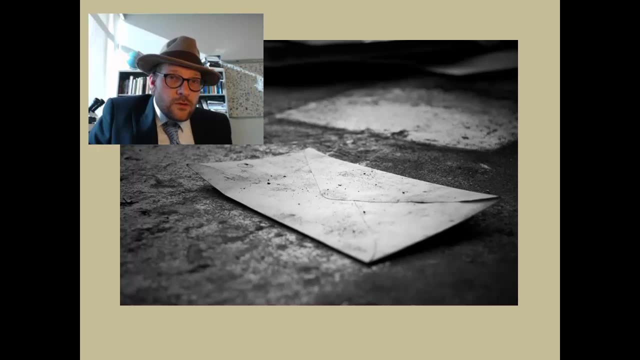 To the idea of spontaneous variation arising from mutations that could arise during the lifespan of an organism. Or maybe there is a modified Lamarck idea where certain traits or characteristics could be passed on once they are gained in the parents. The solution to Darwin's problem lay in a letter that was sent to him, but he never. 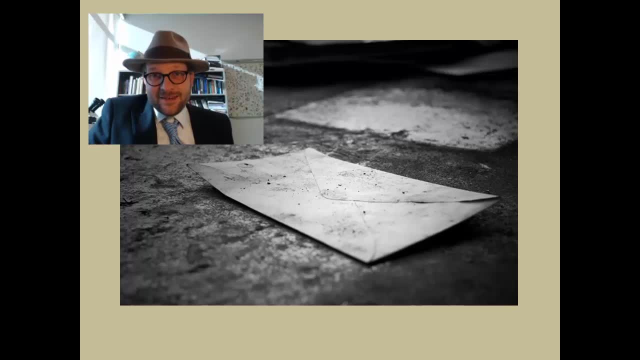 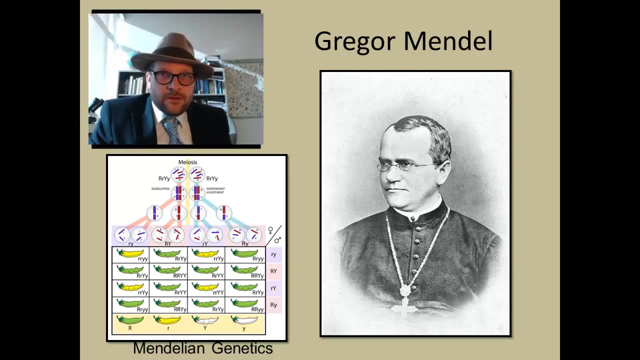 opened it until after he died. We refer to what is in this letter as Neo-Darism, which is a new idea that addressed particularly this problem of variation and inheritance. The letter was from an Agostine friar named Gregor Mendel, from what is today the Czech. 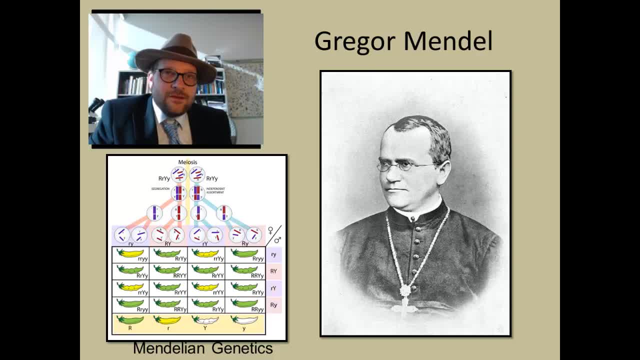 Republic. Mendel is known as the father of genetics. He discovered while growing peas at a monastery that inheritance was not blended but followed a probability distribution. It is much like a game of cards. In a game of cards, the characteristics of each played hand can differ fundamentally. 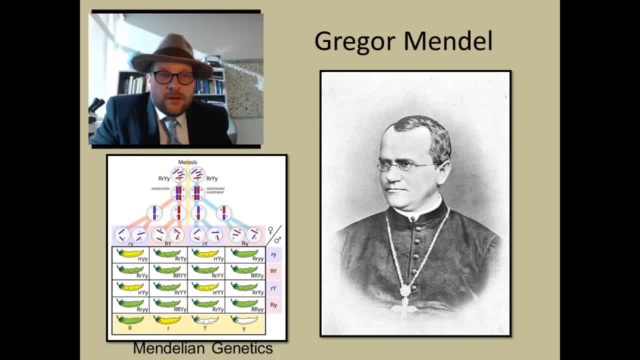 by the interaction of the handful of cards in play to make millions or trillions of different arrangements. Mendel realized that the same reshuffling of characters were happening with his peas By keeping notes on which peas he bred and each generation's expression of those traits. 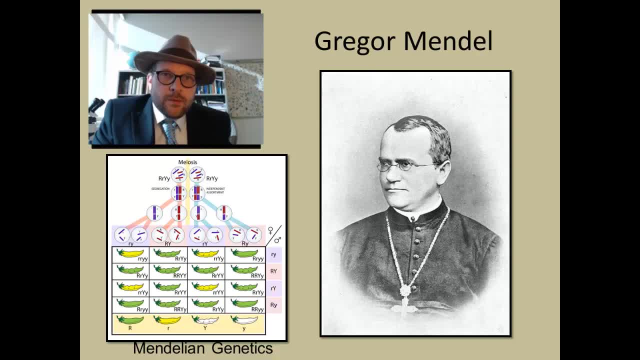 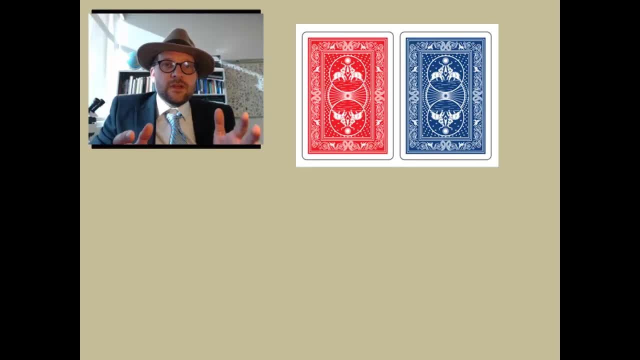 he realized that many characters followed a simple probability distribution. Often a single dominant expression trumps other, less dominant expressions. For example, let's imagine a very simple card game in which there are two types of cards that are dealt. These cards can either be an ace or a king. 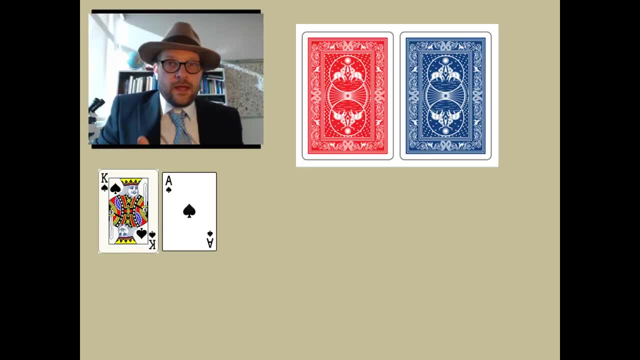 The first random hand has a king and an ace. Another random hand could have two kings. The hand with the different cards has a king and an ace. The hand with the different cards can have two kings. The hand with the different cards can have two kings. 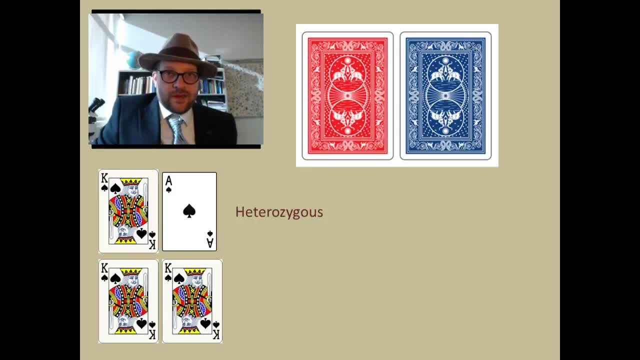 Another possible random hand is called heterozygos, and the one with the same cards- a pair- we would call homozygos. There are two other possible hands in our game: One with a pair of aces and one with a pair of aces in the first card and a king in the. 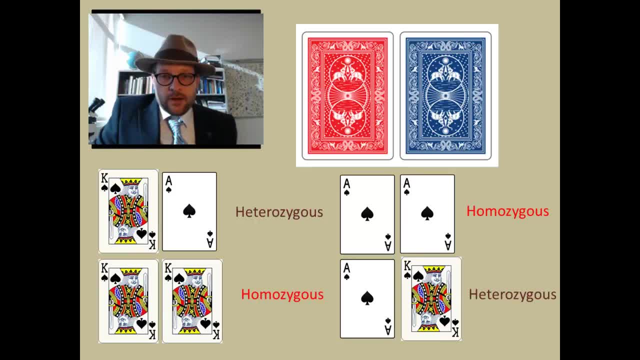 second card: Both a homozygos and a heterozygos. Note that if inheritance follows this, randomness variation will be maintained, but on average, 25% of the hands will have two aces. On average, 25% of the hands will have 2 aces. 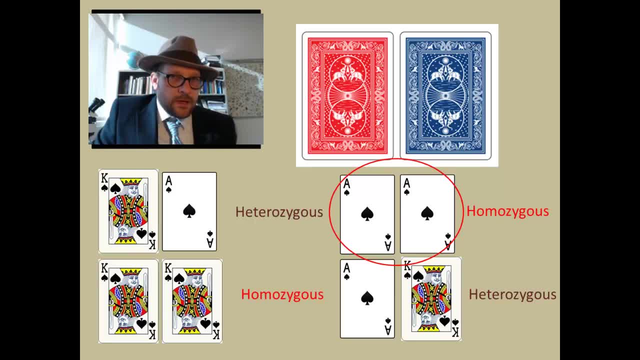 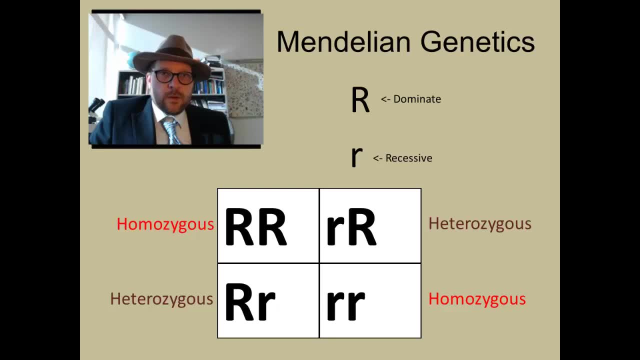 This could code for a particular characteristic, like peapod color, for example. In Mendelian genetics a Putnam square is used to explain the simplest card game in which you have two types of cards. in this case we have a big R and a little r. 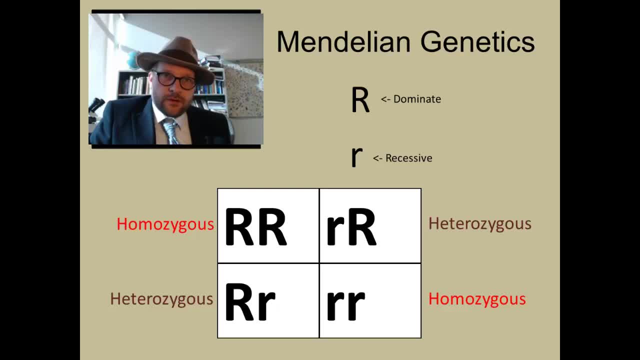 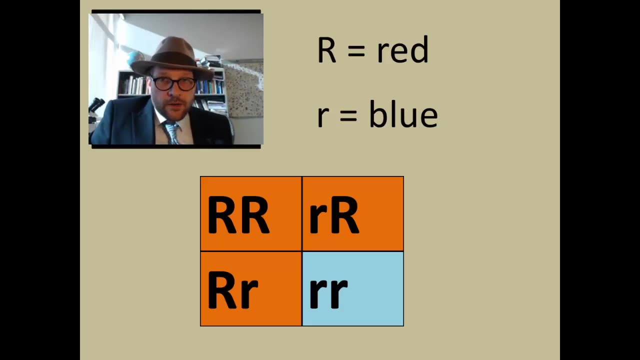 The big R is the dominant character and will express itself whenever it is played in the offspring. The little r is recessive and only expresses itself in the absence of the big R, If the big R codes for a red color and the little r codes for an expression of a blue color. 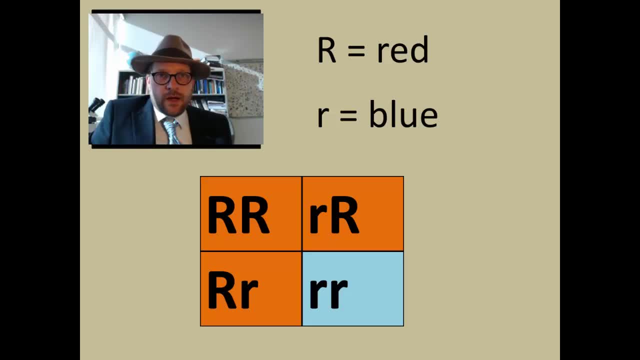 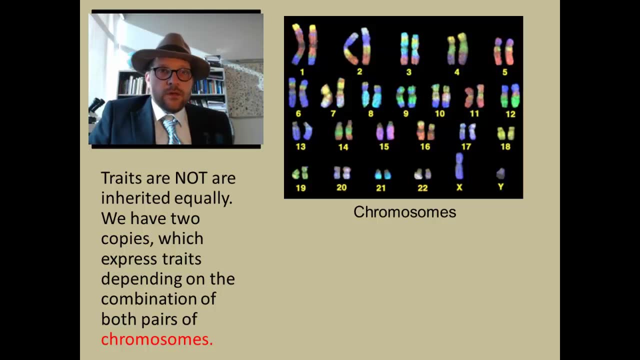 the probability that an offspring has a blue color is only 25%. The discovery Mendel made was that sexually reproducing organisms have paired chromosomes. These chromosomes split, with one side originating from the mother and the other side originating from the father. Every cell has a copy of the chromosomes in the nucleus, and chromosomes are made up of. 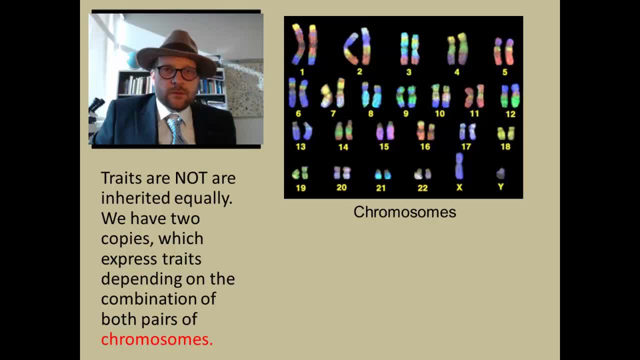 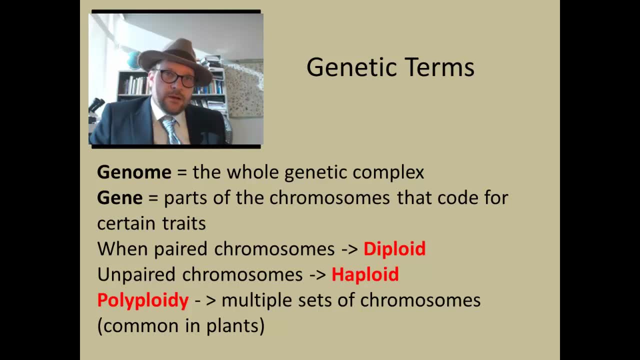 DNA. Let's quickly define some key terms. A genome is the whole genetic complex. A gene is the parts of the chromosome that code for certain traits. When chromosomes are paired, we call that a diploid. When chromosomes are unpaired, we call that a haploid. 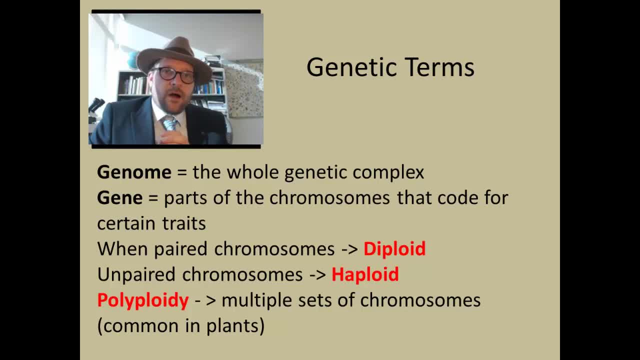 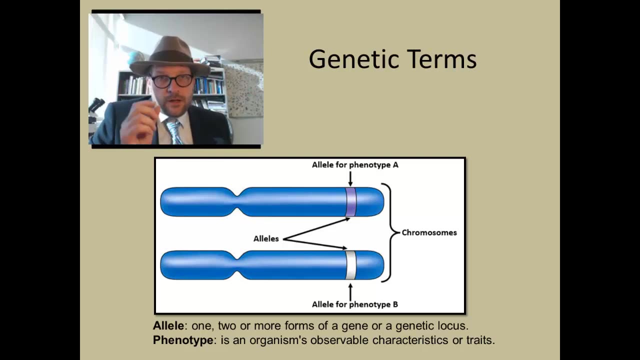 A polypoid or polypoidally are where you have multiple sets of chromosomes. This rarely happens in animals but is very common in plants, and we will talk more about that later on. An allele is where you have one, two or more forms of a gene or genetic locus on a chromosome. 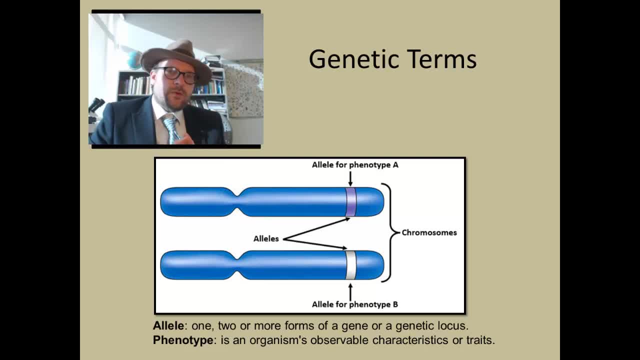 A phenotype is the organism's observable characteristics or traits that are coded for by that allele. In paleontology we can refer to fossils' phenotype, the expression of the trait, but never the gene allele or genome, which are not preserved. Each chromosome is made of different genes. 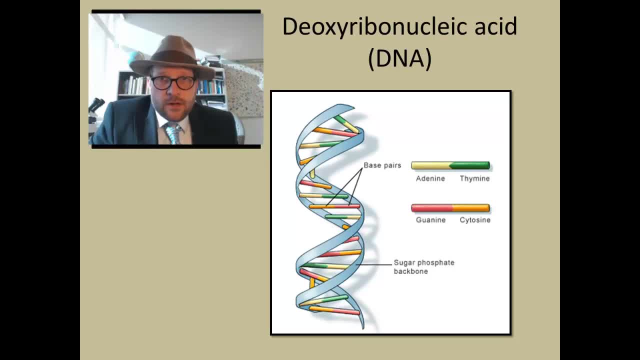 Each chromosome is made of different traits. Each gene is made of dioxyribonucleic acid, a single complex string of four base pairs: adaline, thymine, guanine and cytosine. DNA serves as the blueprint for RNA. 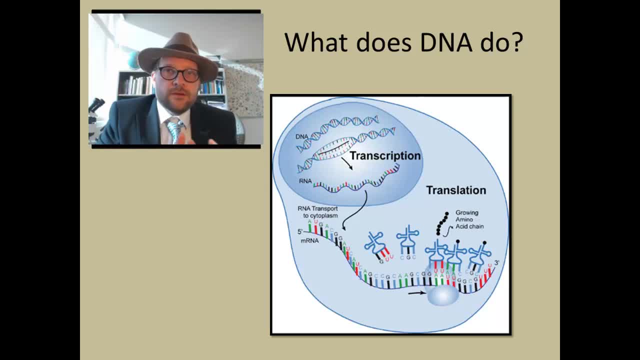 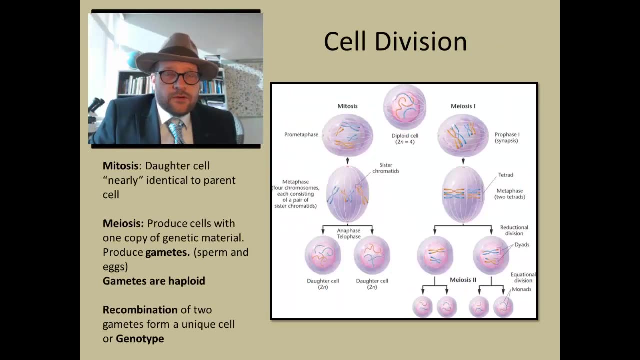 RNA is like a Xerox copy of the DNA strand and is sent into the cell from the nucleus, where amino acids form complex proteins along the surface of the RNA. These proteins facilitate the growth and function within the cell. There are two types of cell division that can happen. 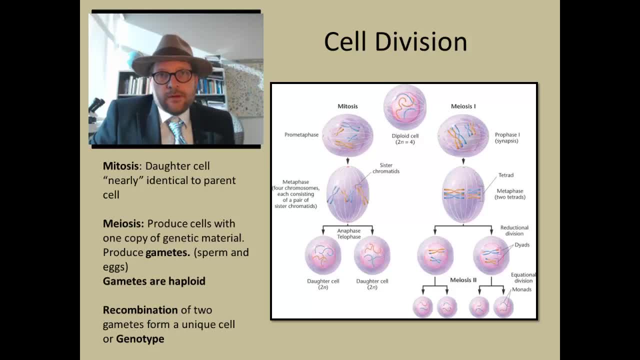 The first is mitosis. Mitosis is where you have a daughter cell that is nearly identical to the parent cell. This is what happens in asexually reproducing organisms. The chromosomes remain the same. It also happens in all multicellular organisms with cell division within a single individual. 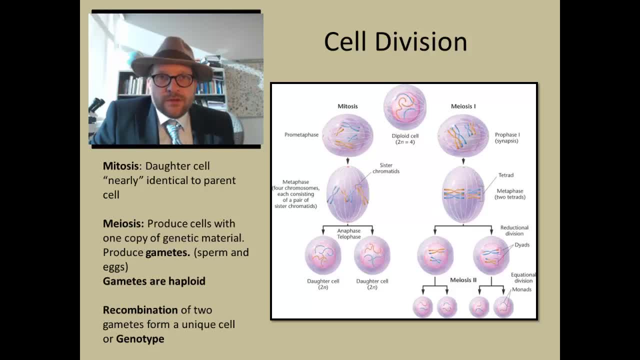 Many bacteria exhibit this type of reproduction as well, although there is a significant advantage to sexual reproduction because it quickly mixes variation across a population and can speed up the reaction to natural selection. The second type of cell division is meiosis. Meiosis is where you have produced cells with one copy of the genetic material. 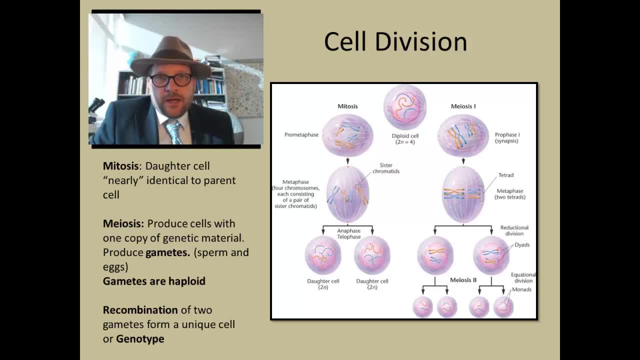 Meiosis produces what are called gametes. these are the sperm and eggs. Throughout the semester, we will be talking about gametes, in which many invertebrate groups and plants can exhibit their own life within a complex cell. In most animals and plants, these are the reproductive cells, the sperm and eggs. 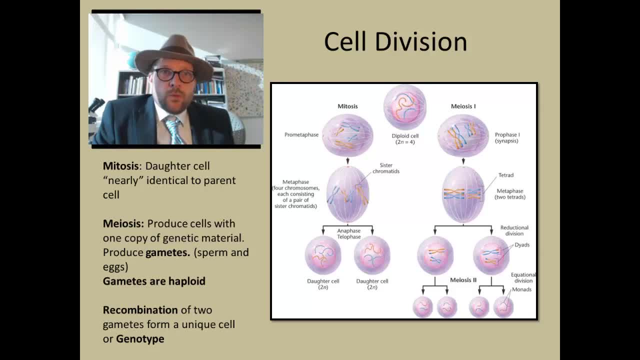 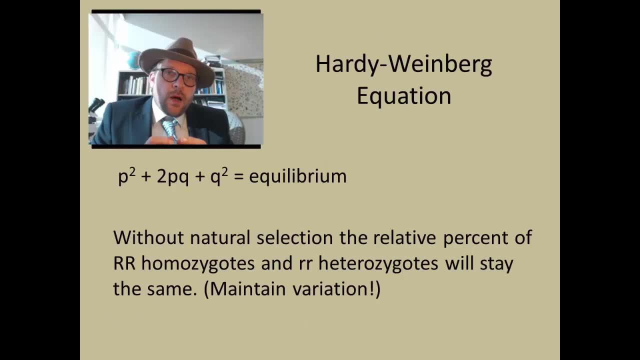 Gametes are haploid, which means they have one set of chromosomes. Recombination of two gametes form a unique cell or genotype which have paired chromosomes. The probabilities of each outcome in a diploid chromosome can be expressed with a simple mathematical formula called the Hardy-Weinberg equation, where the P and Q are the allele. 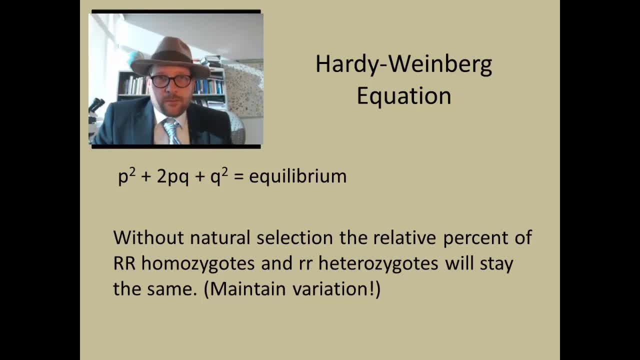 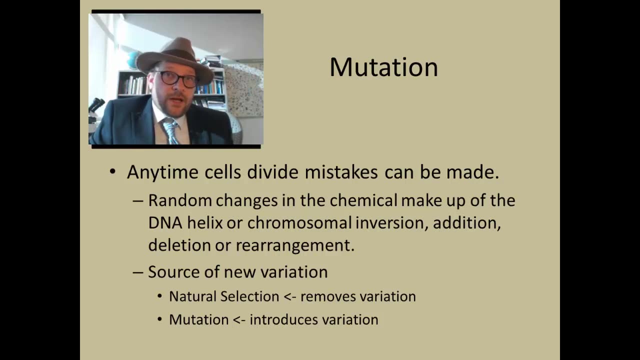 frequencies for each trait. Hence, as organisms mate, variation is maintained in the population and hence natural selection can work on this variation. Yay, Darwin's problem has been solved. Mutation is still a common way to introduce variation, because every cell is replicated millions and trillions of times, leading to the introduction of errors. 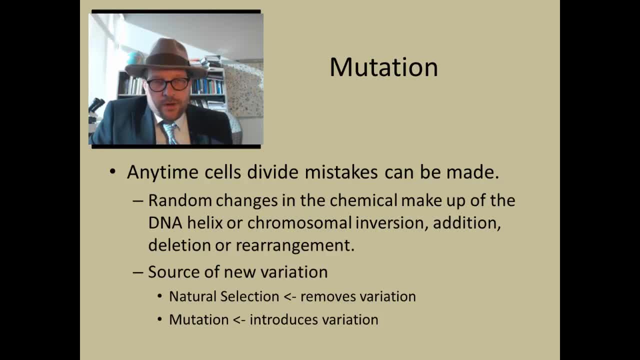 Random changes in the chemical makeup of the DNA helix. Homozyme. inversion, addition, deletion, rearrangement are the source of new variation. So natural selection removes variation in the population, mutations introduce new variation and sexual mating maintains variation in the population. 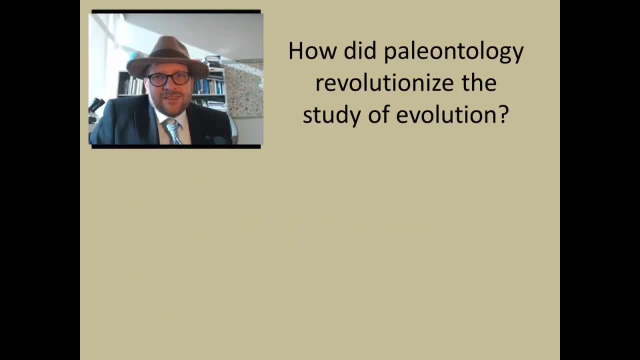 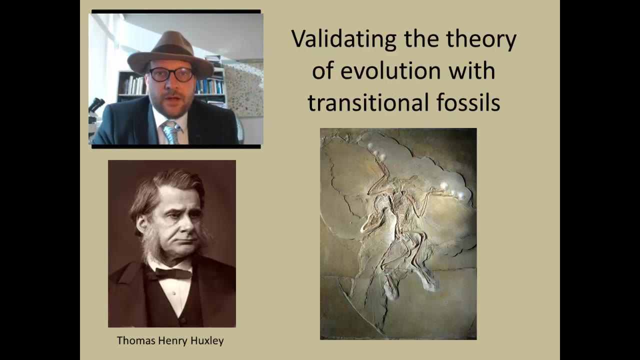 What about fossils? All this study of evolution does not seem to involve paleontology. How did paleontology revolutionize paleontology? I will explain why. Paleontology did this in three major phases. First, paleontology validated the theory of evolution with numerous transitional fossils. 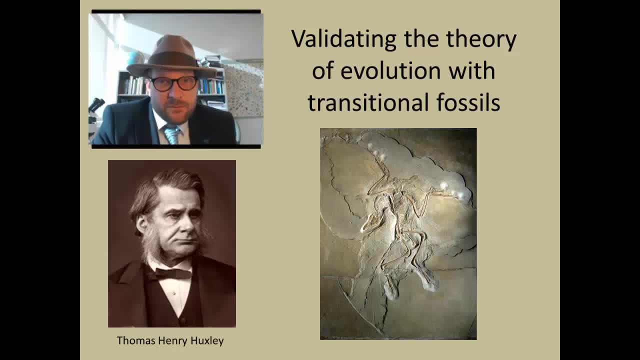 After Darwin published the origin of species, the fossil record started to get much better. In 1849 only four species of dinosaurs were known, but by 1900, hundreds of dinosaurs were discovered, a complex bush of extinct creatures, The first published specimen of Archaeopteryx. 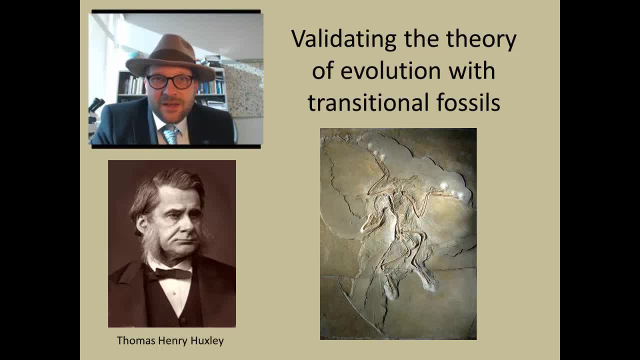 Archaeopteryx. Archaeopteryx was only discovered two years later, which meant that Darwin, in later additions, was able to comment about his discovery. In fact, Thomas H Huxley's work on the origin of birds strongly vindicated Darwin's idea. 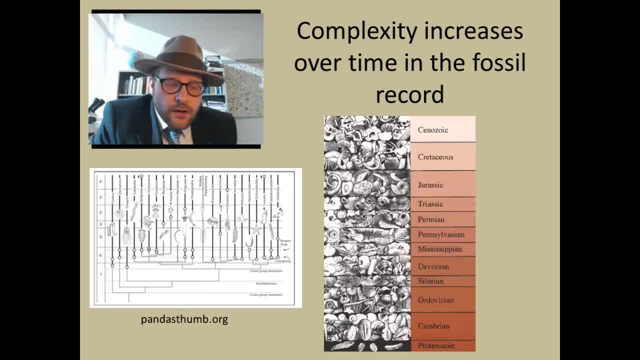 that organisms change through time. Early on. paleontology also showed that complexity increases over time in the fossil record. This validation of evolution is the strongest line of evidence for evolution. Lower, older stratigraphic units have less complex organisms. Informationen we get about evolution show that theé이w cannot coexist in tissue. we see: 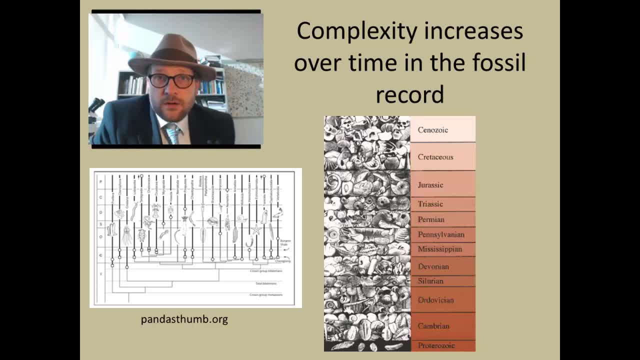 no Templinia easy to see. theídoine that we find were Depot daha al deeper in parcels of rocks, as Wood 시청 found on Mes Sunday organisms, while younger, higher stratigraphic units contain more complex organisms. This is the foundation of geology, as well as a strongly, continually tested notion of 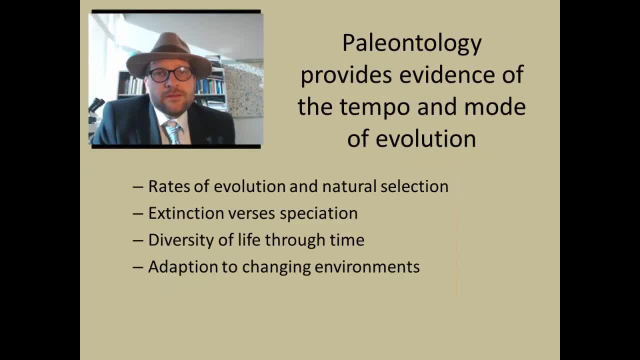 evolution. Paleontology also provides evidence for the tempo and mode of evolution, or how fast or slow organisms change, and the style of those changes. These key questions were addressed viciously in the 1970s and 1980s. In the next lecture we will explore evolutionary rates more closely. but paleontology revolutionized. 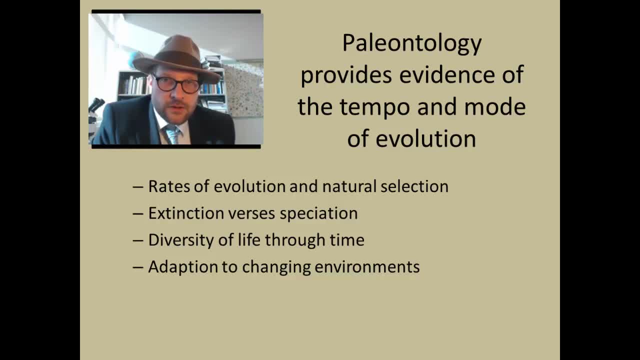 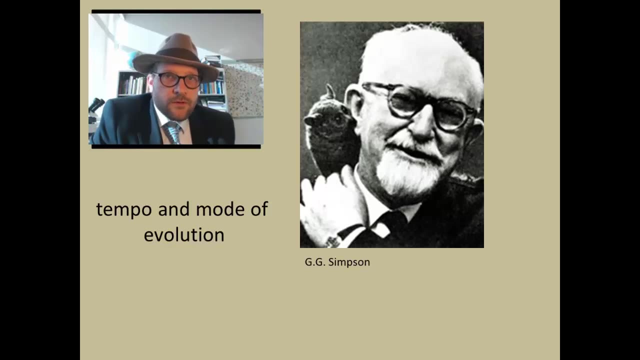 our understanding of the rates of evolution and natural selection, the patterns of extinction and speciation, the diversity of life through time and the adaptation of organisms to a changing Earth in its changing environment. The terms tempo and mode come from the classic book by the paleontologist GG. 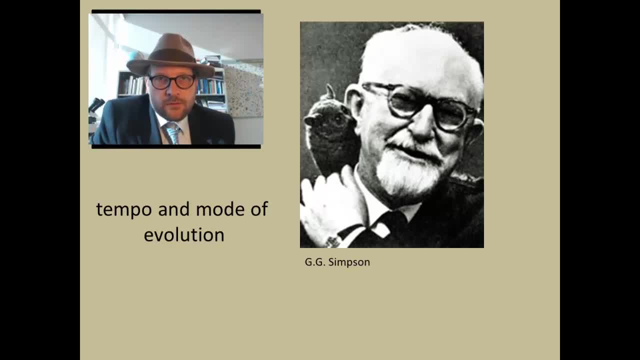 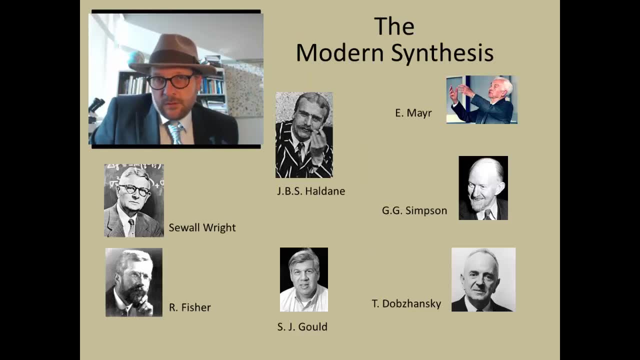 Simpson, entitled Tempo and Mode in Evolution, published in 1945.. GG Simpson was part of a group of evolutionary scientists who studied evolution from a multidisciplinary approach which included paleontologists, geneticists, biologists, embryologists and. 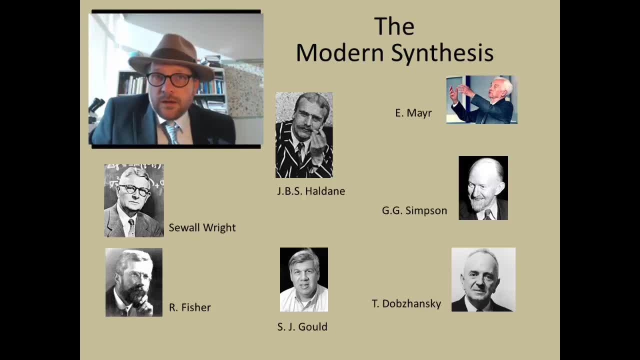 others that looked at evolution using different lines of evidence but widely met and read each other's work. Sadly, paleontologists are not often included in many discussions of evolutionary science, as molecular biologists have monopolized the study of evolution using a molecular approach. 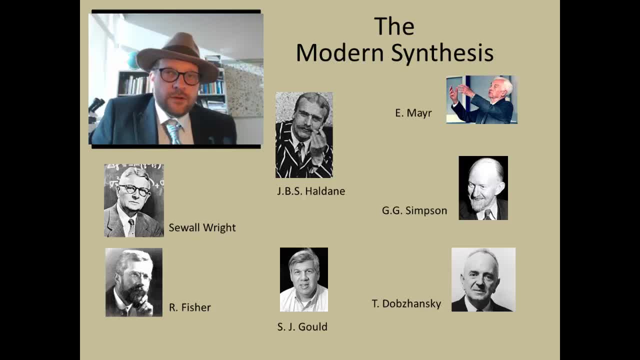 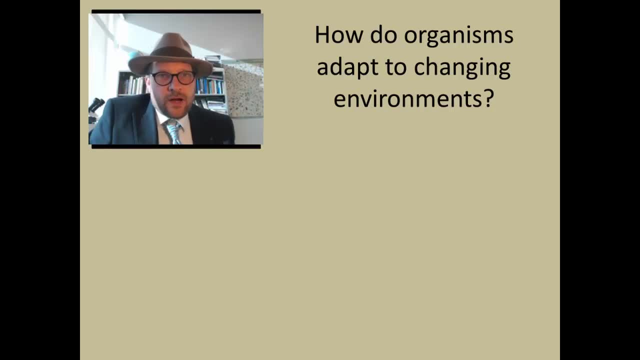 The key question is: what is evolution? The questions in evolution can only be answered using the fossil record, and these include: 1. How fast is evolution? 2. How do organisms adapt to changing environments? 3. How common is extinction? 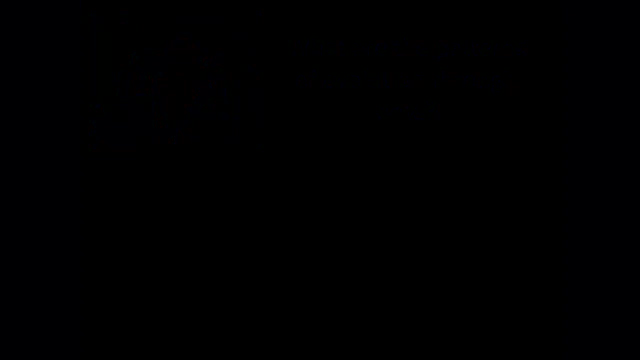 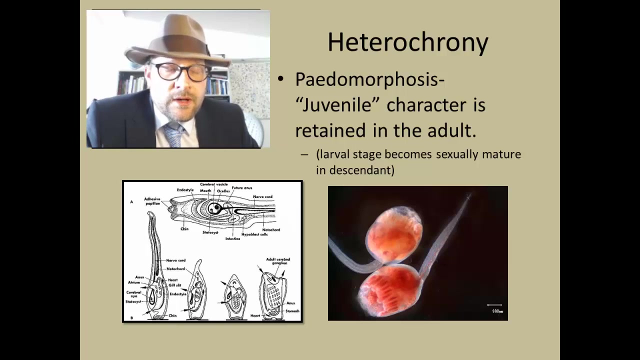 4. What are the patterns of evolution through time? I want to talk quickly about something I didn't mention when we talked about ontogeny, and that is this term called heterochrony, which means different time. The first example I'm going to use is called pedomorphism. 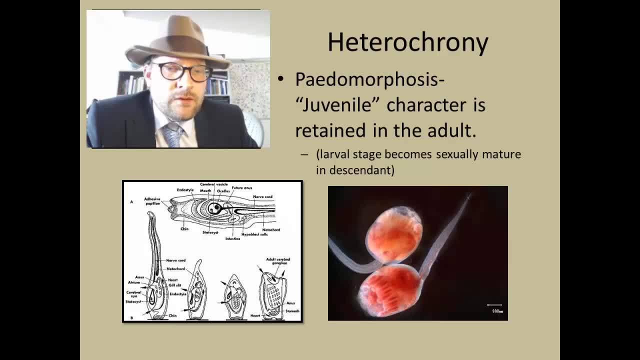 Pedomorphism is where a juvenile character is retained in the adult. A good example of this is probably with tunicates in paleontology. Tunicates are a group of organisms that have a larval stage, that have a mobile tail, that swim around in the water column.